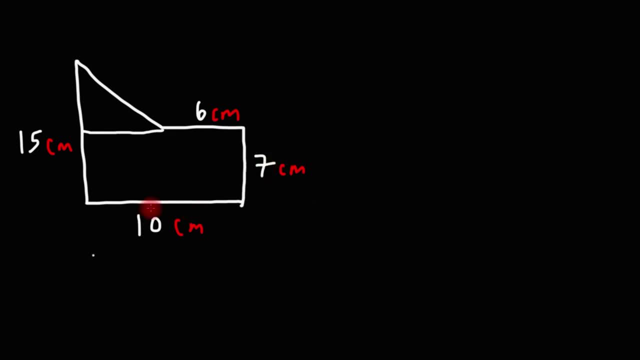 10 times 7.. So that's going to be 70, with the units square centimeters. Now let's focus on the triangle. What is the length of the base of the triangle? Notice that it's the difference of these two numbers. If we subtract 10 by 6, we're going to 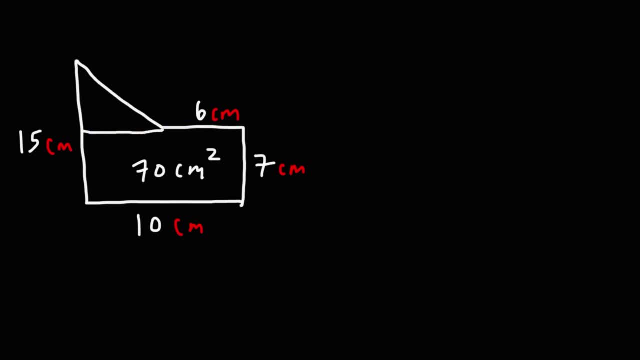 get the amount left over, which is going to be 10 times 7.. So we're going to get the amount left over, which is going to be 4.. So this is 4 units long. Now, what about the height of this triangle? 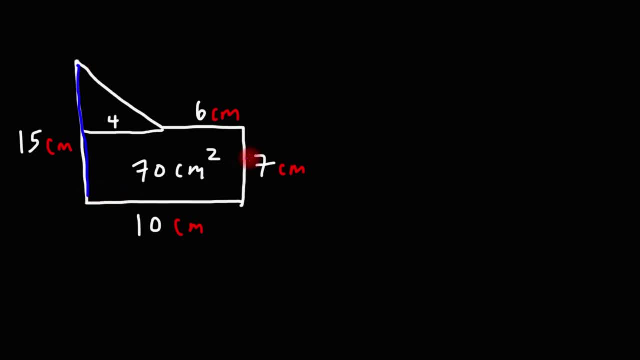 Notice, this side is 15 units long, or 15 centimeters, and this side is 7.. Subtracting those two will give us this portion, So it's 15 minus 7, which will give us 8. So we have a. 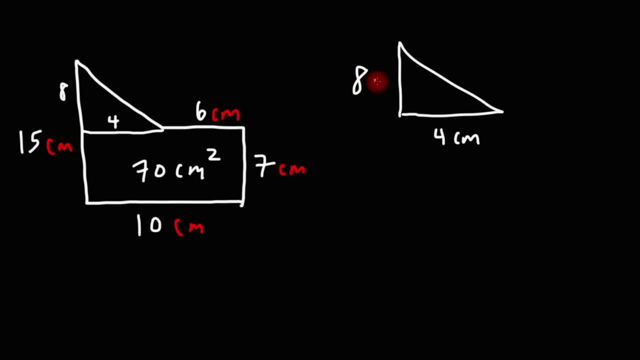 triangle with a base of 4 centimeters and the height of 8 centimeters. So using the formula one half base times height, it's one half 4 centimeters times 8 centimeters. 4 times 8 is 32.. Half of 32 is 16.. So this part is: 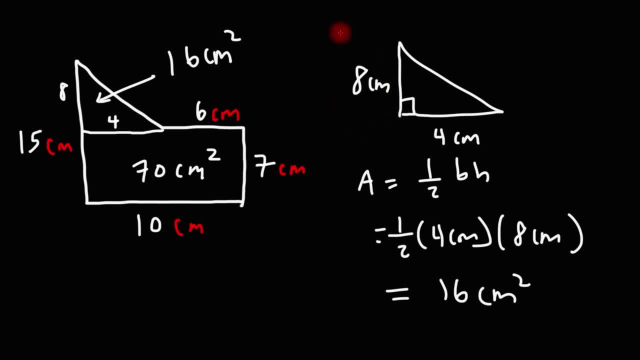 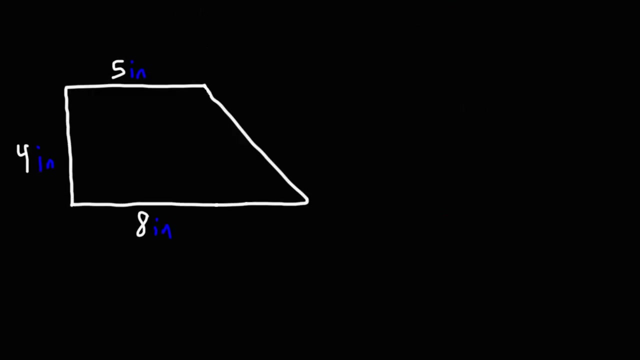 16 square centimeters. So now we can calculate the total area by adding those two values: 70 plus 16 is 86. So that is the area of that particular composite figure. Now let's work on this problem. Let's find the area of this composite figure. 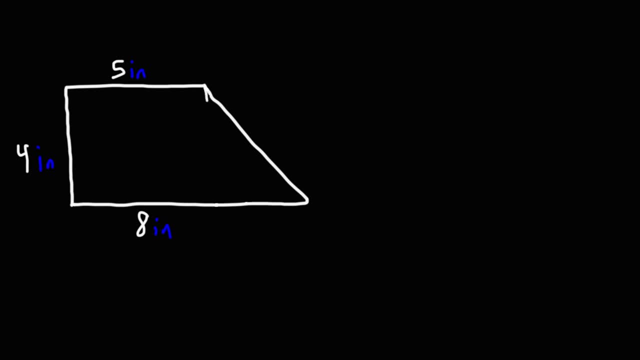 What I recommend doing is drawing a line right here to separate this into a rectangle and a triangle. Now to find the area of the rectangle, it's just going to be the length of 5 inches times the width of 4 inches. 5 times 4 is 20.. 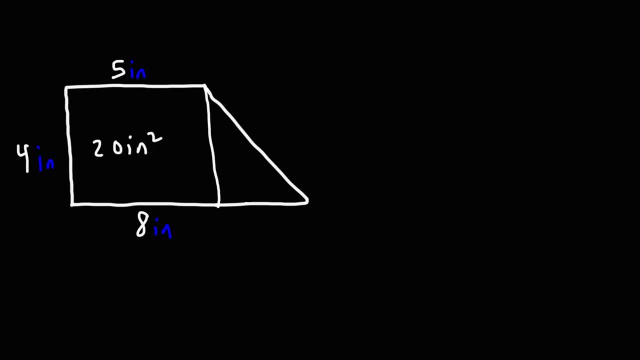 So we're going to get 20 square inches. Now let's focus on the triangle. We need to determine the height of the triangle and the base For the height we could see. it's the same as this side, which is 4 inches. 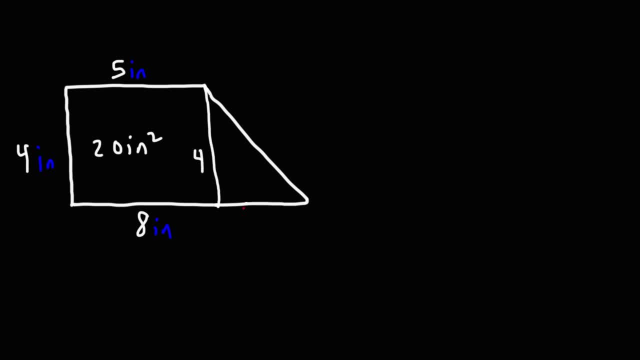 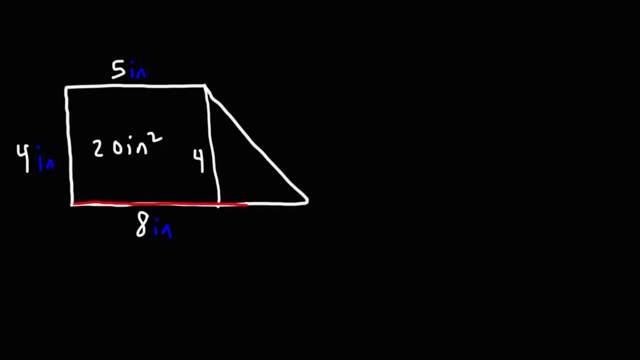 How long is it? Now we know that this segment is 8 inches and this segment is 5.. So the difference between these two numbers will give us the length of the base. So it's 8 minus 5, which is 3.. 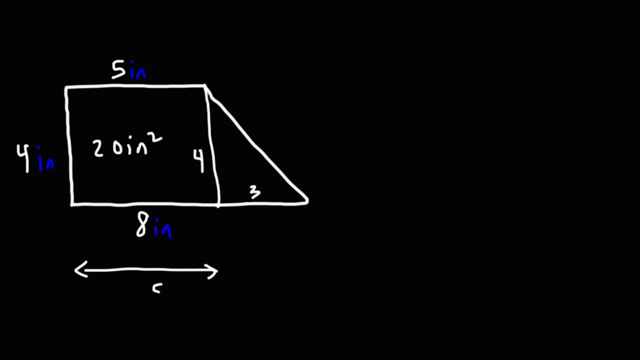 And if you want to visually see it, we know this part is 5,, this part is 3, and that will give us the total length of 8, which is what we're going to get, And that will give us the total length of 8, which is what we have here. 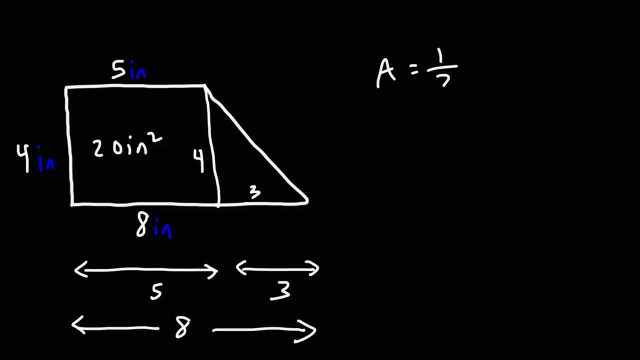 So now we can calculate the area of the triangle. It's 1 half base times height. The base is 3,, the height is 4.. 3 times 4 is 12, and half of 12 is 6.. So the area of the triangle is 6 square inches. 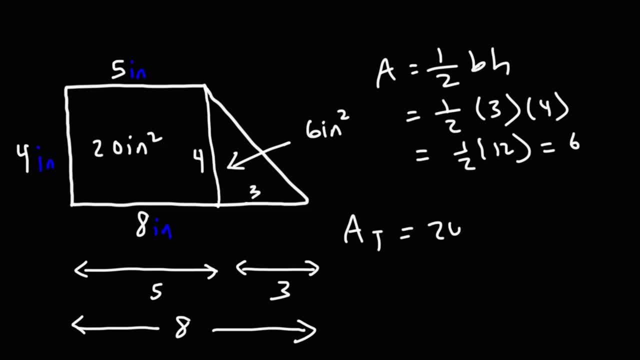 So now we can calculate the total area of the composite figure. It's going to be 20 square inches plus 6 square inches, and that will give us a total of 26 square inches. So that's the area of this particular composite figure. 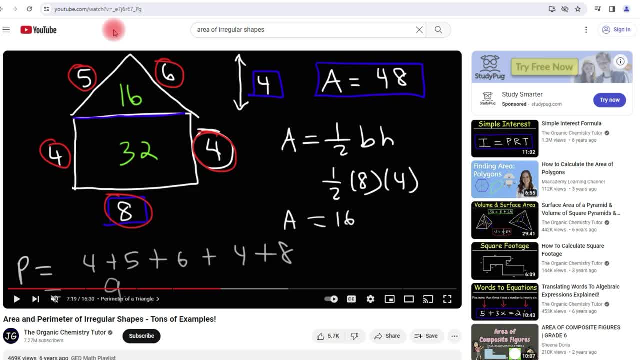 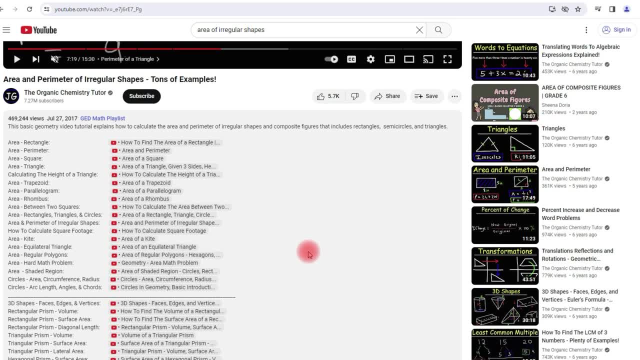 Now, for those of you who want to find other related content, feel free to check out the links in the description section below, So you can find it by clicking on More. and I have other videos, like how to find the area of a trapezoid. 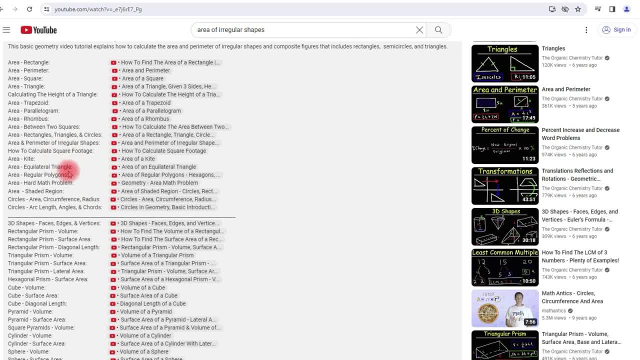 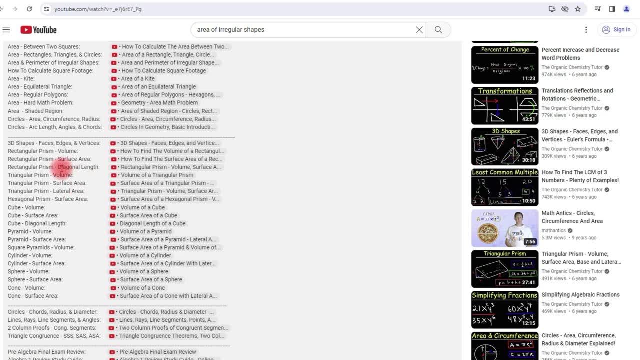 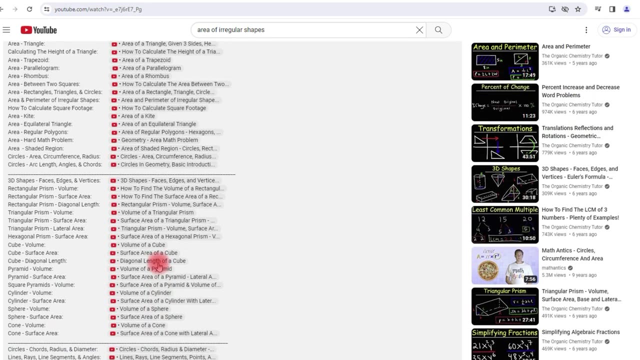 a parallelogram, a rhombus, a kite, an equilateral triangle, and also how to find things like volume, surface area, a rectangular prism, a triangular prism and other shapes. So feel free to take a look at this when you get a chance. 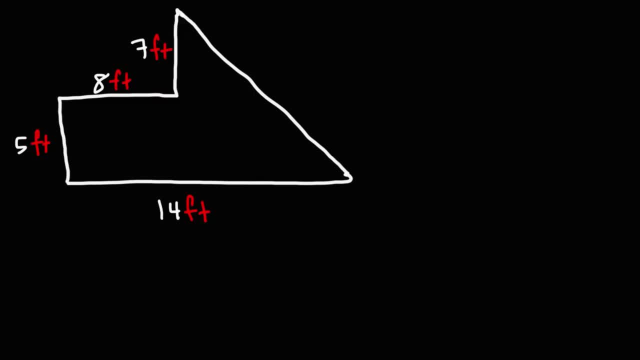 for those of you who are interested in that. Now let's work on this example For this problem. I'm going to draw a line right here to make it into a triangle. So I'm going to draw a line right here to make it into a triangle. 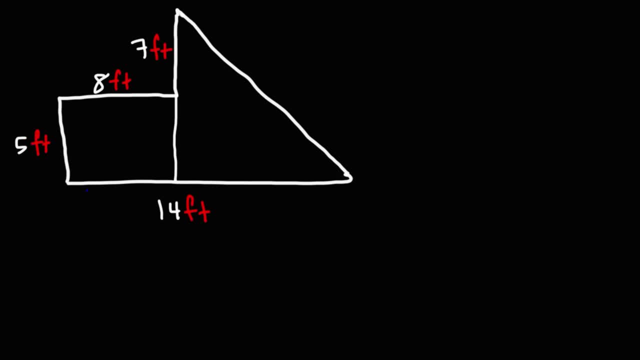 So I'm going to draw a line right here to make it into a rectangle and a triangle. For the rectangle, we can see that we have a length of 8 and a width of 5.. So 8 times 5, that's going to give us an area of 40 square feet. 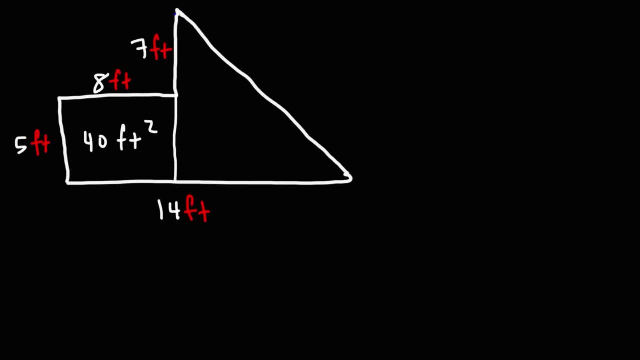 Now let's focus on the triangle. We need to determine the height of the triangle and the length of the base. If we focus on the triangle, If we focus on the height, we can see that it's the sum of this part and this part. 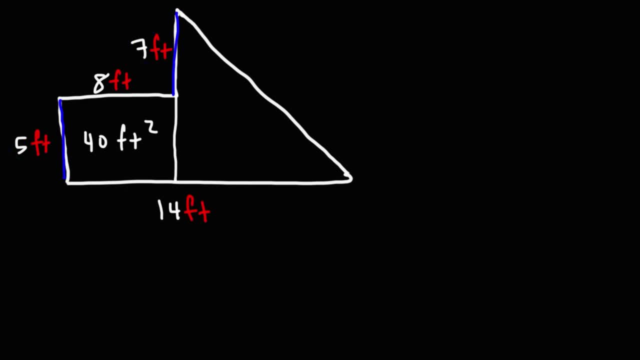 So it's 7 plus 5,, which is 12.. So I'm just going to redraw it over here, So we have a height of 12.. Now let's focus on the left of the base. This part here is 14.. 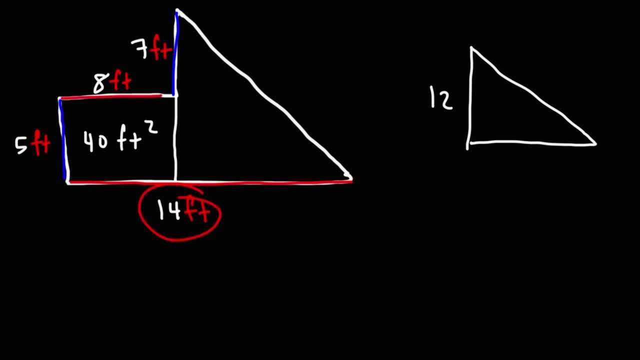 This part is 8.. If we subtract the total of 4,, we'll get the total of 14 by 8. We'll get the difference, which that's going to be 6.. And this picture is not drawn to scale, just in case you were wondering. 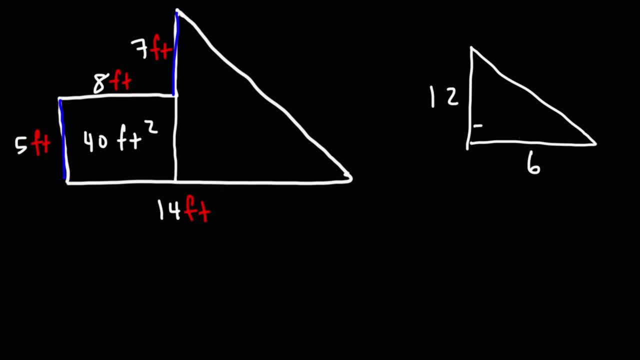 So this is 12,, this is 6.. And now we can calculate the area. So the area is going to be 1 half base times height. The length of the base is 6.. The height of the triangle is 12.. 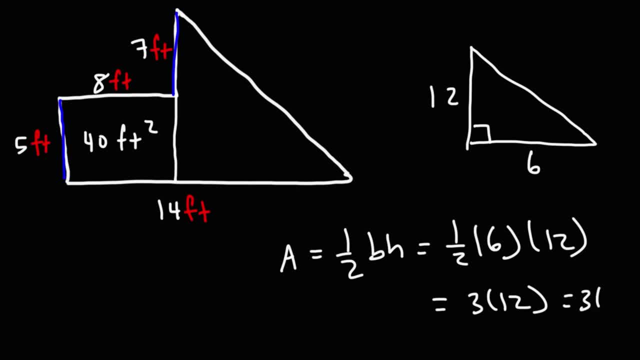 Half of 6 is 3. And 3 times 12 is 36.. So this part is 36. Square feet, And again, this is not drawn to scale. as you can see, The total area is going to be 40 plus 36.. 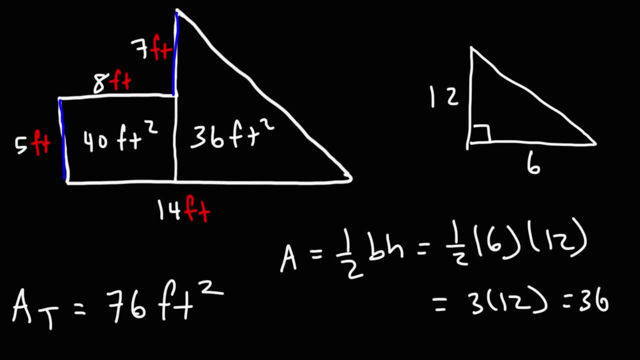 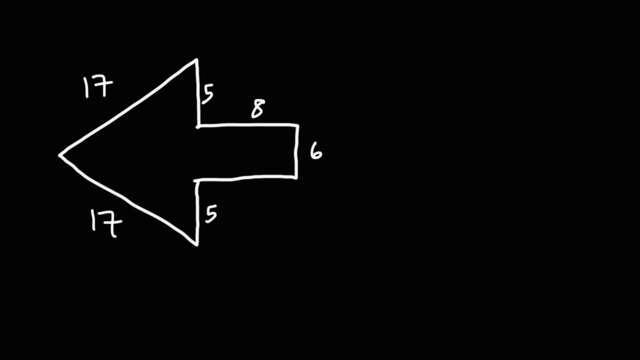 So for the composite figure, the total area is 76 square feet. Now let's work on this example. So we want to find the area of basically an arrow. How can we do this? Well, it might be helpful if we draw a line there. 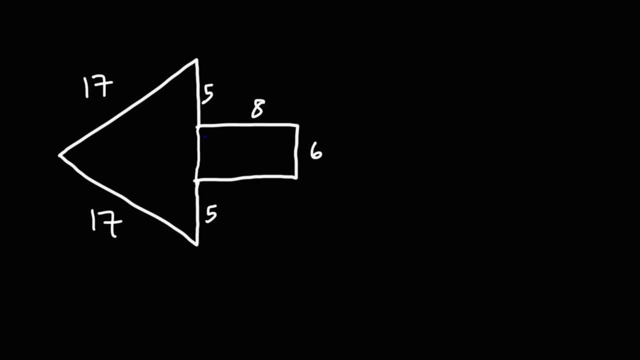 So we have a rectangle with a length of 8 and a width of 6.. So 8 times 6, that's going to be 48 square units. Now what can we do to find the area of that triangle? Notice that these two are the same as those two. 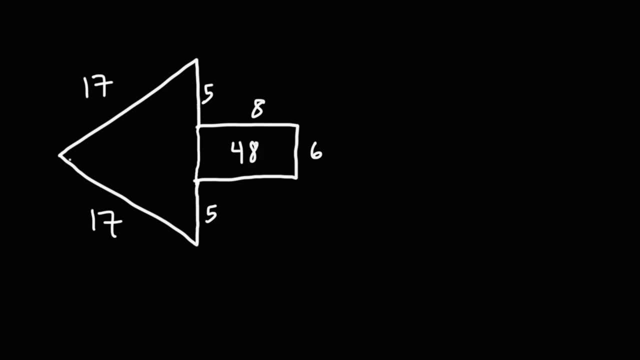 So if we draw a line right in the middle, we can create two equivalent triangles. Now what we need to do is determine the height of the triangle. If we can figure what h is, we can get the answer. Now, this point here is going to be the midpoint of this segment. 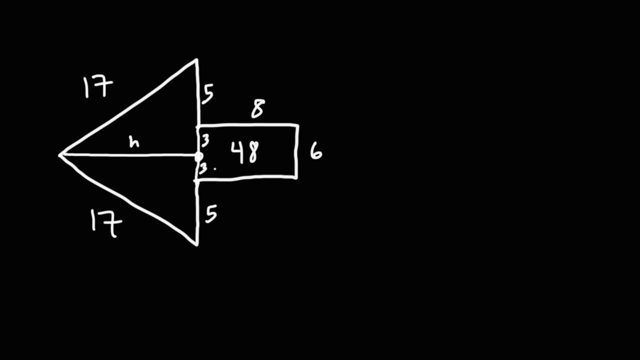 So that's going to be the midpoint of this segment. So that means that this side, this point, is 3, and this portion here is 3.. So notice what we have. Let's draw the top triangle. We want to calculate h. 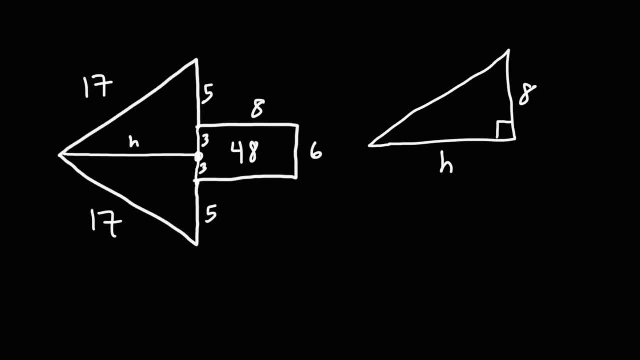 This is 8, and this is the right triangle, and the hypotenuse is 17.. So we could use the Pythagorean theorem. Let's call this a, b and c. a squared plus b squared is equal to c squared. 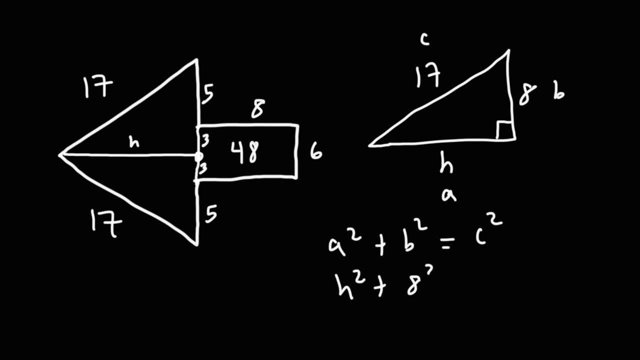 a is the same as h, which is what we're trying to find. b is 8,, c is 17.. 8 squared, or 8 times 8, is 64.. 17 squared, which is you're multiplying two 17s together. 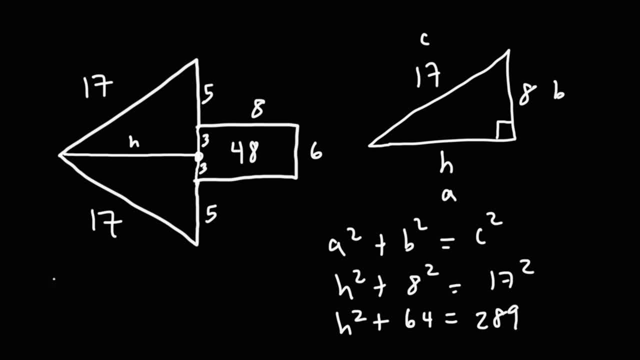 17 times 17 is 289.. To get h squared we need to subtract 289 by 64. So 289 minus 64 is 225.. And to calculate that we need to subtract 289 by 64.. To calculate h we need to take the square root of both sides. 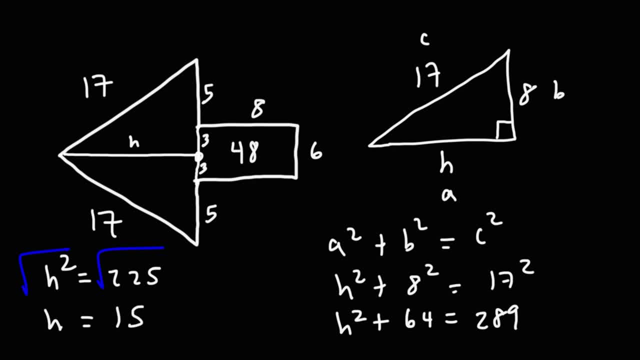 The square root of 225 is 15.. So h is 15.. If you know your special right triangles, you can quickly determine this answer. There's a 3,, 4, 5 right triangle. There's the 5,, 12, 13 right triangle. 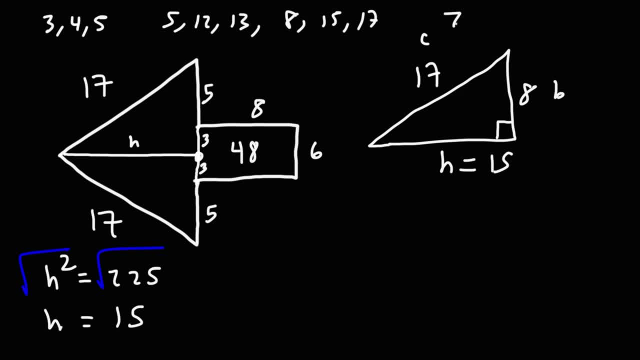 There's the 8,, 15,, 17 right triangle And there's also the 7,, 12,, 13 right triangle, And there's also the 7,, 12,, 13 right triangle, And there's also the 7,, 12,, 13,, 24,, 25 right triangle. 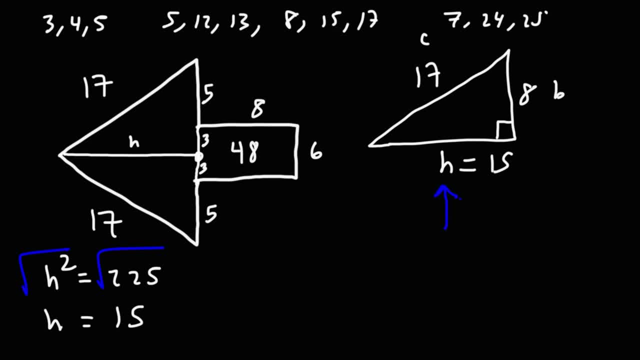 So if you know these numbers, you can easily determine that the height will be 15.. If you have a right triangle where one side is 8, the other side is 17,, the missing side will be 15.. So now let's go ahead and finish this problem. 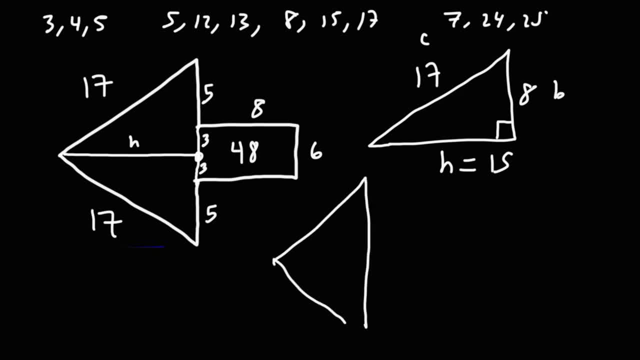 So let's focus on the large triangle. The height of this triangle is 15.. And if we look at the left of the base, it's going to be 5 plus 5,, which is 10, plus 3 and 3..